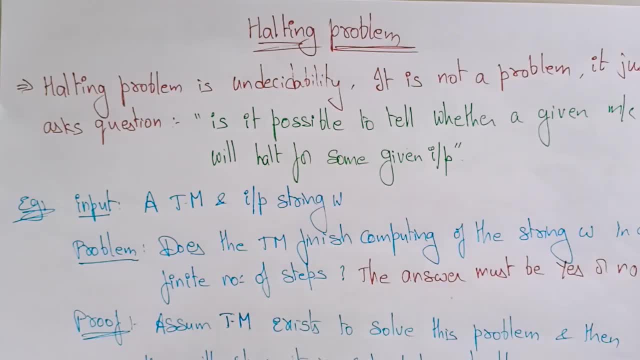 Hi students, welcome back Now. coming to the next topic in the theory of computations, that is a halting problem. By reading this name, you get an idea that halting means we are stopping that problem. Okay, so when you are stopping that problem, when you are halting that problem Now. 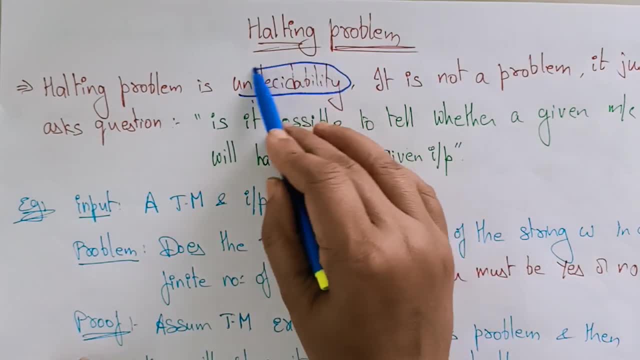 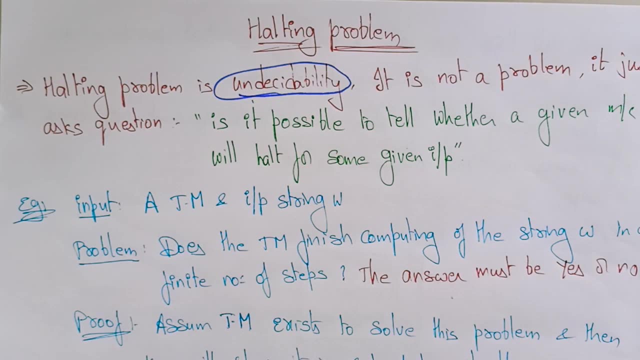 let's see, The halting problem is undecidability. So whenever you are not able to decide whether the input or whatever the output that you get, you are not able to decide that then you in that case you will halt. that problem Means it is not completely covered. The halting problem is: 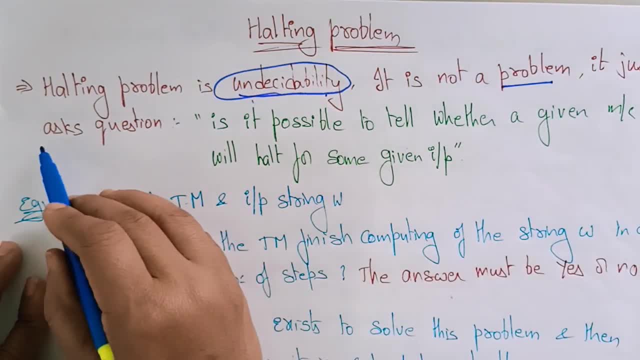 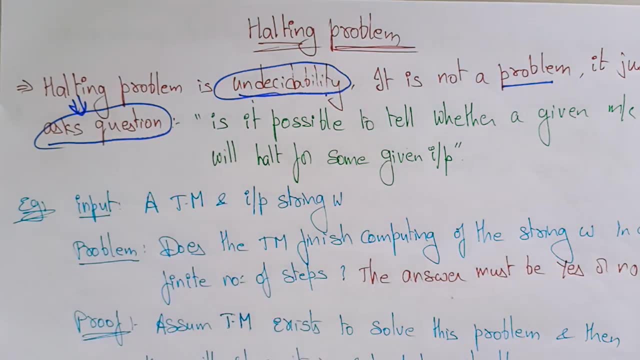 undecidability. It is not a problem, It is just ask the question. So this is a main difference. You don't think halting problem is a problem. It is actually. it is not a problem, It's just asking a question. The halting problem is saying: is it's asking the Turing machine a question? 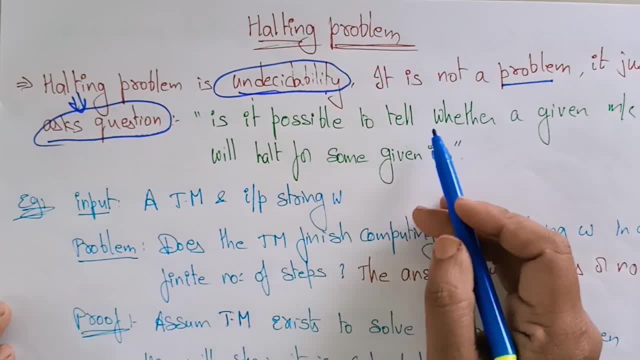 What type of question it is asking. Is it possible to tell whether a given machine will halting? Halt for some given input means it is asking: is whatever the is it possible to tell whether a given machine, whatever the machine Turing machine we are taking, will halt for some given input only? 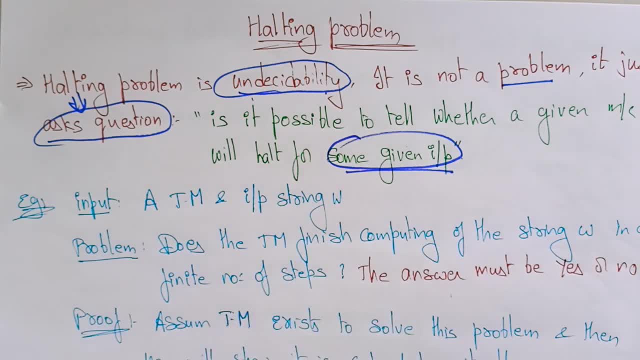 for some given input, not for completely. So whatever the input you are given. So for that input I'm not getting the answer is there is any possible to halt that input? So it's just asking the question. that is a halting problem. 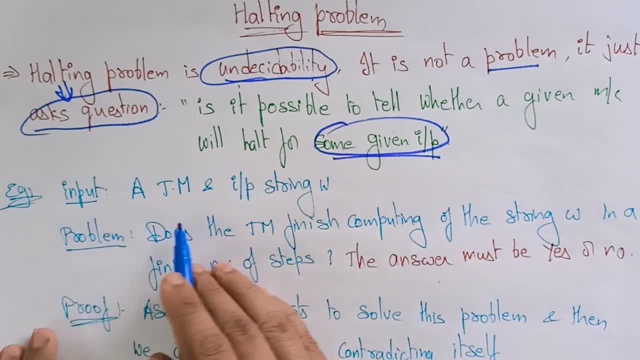 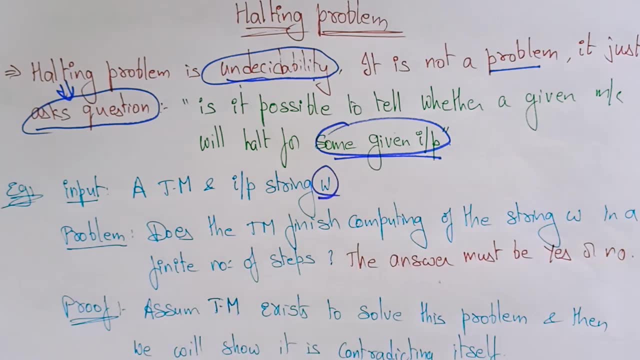 Let me explain you the example. Suppose if I taken an input, a Turing machine input of string w Okay. take in some input string w Okay, W, consisting of some alphabets, input symbols. Now the problem is: does Turing machine finish? 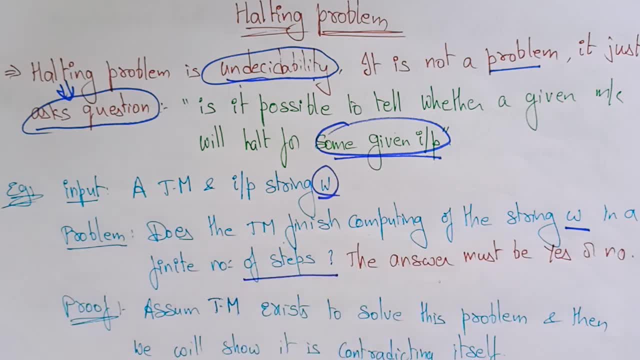 computing of a string w in a finite number of steps. I don't know whether it finished or not. Okay, I'm having a problem that does a Turing machine is complete finish computing the w string, whatever the w string of the string of the string. So I did a Turing machine, I encapsulated the strings。 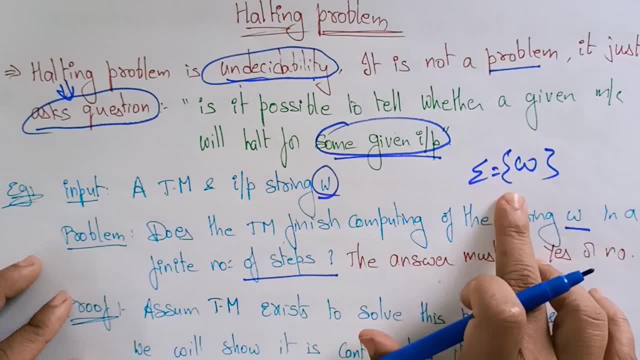 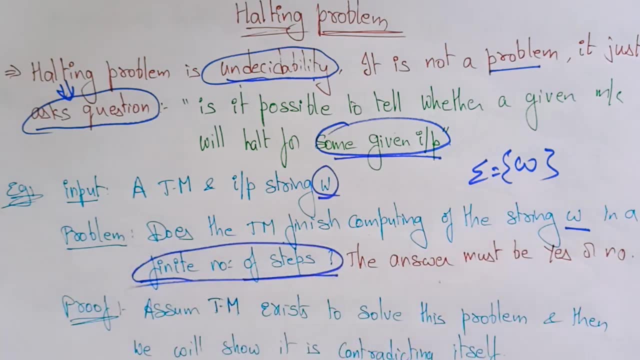 string i have taken is that come finish the computing of the string w in a finite number of steps. in a finite number of step, the answer must be s or no, because undecidable. i'm not able to tell whether it complete the string in a finite number of steps or i don't know. so the answer for 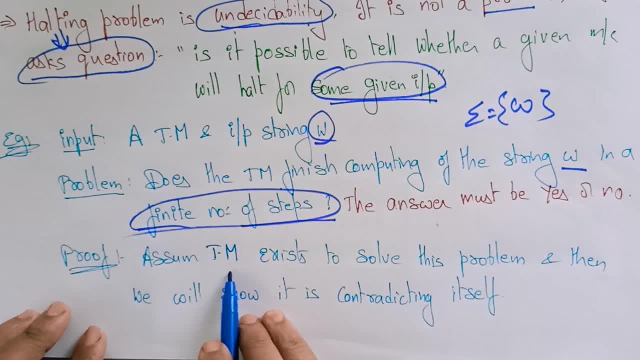 this means yes or no? now let's see the proof. assume turing machine exists to solve this problem. let us start start with the positive thinking. let us assume that turing machine exists to solve this problem. it is solving this problem and it is computing the string in a finite number of steps. 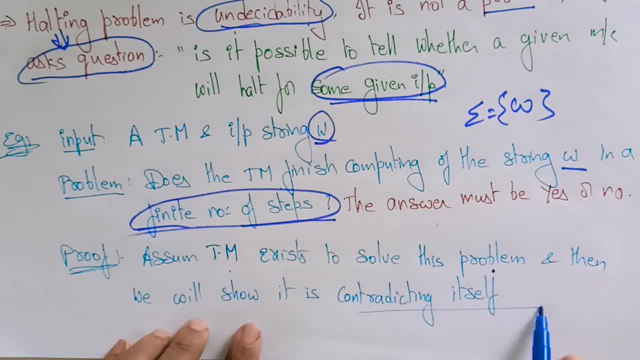 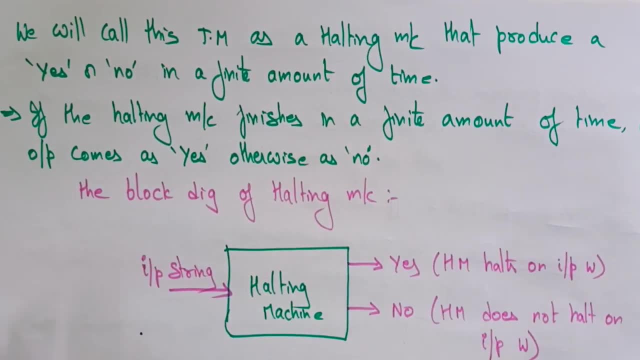 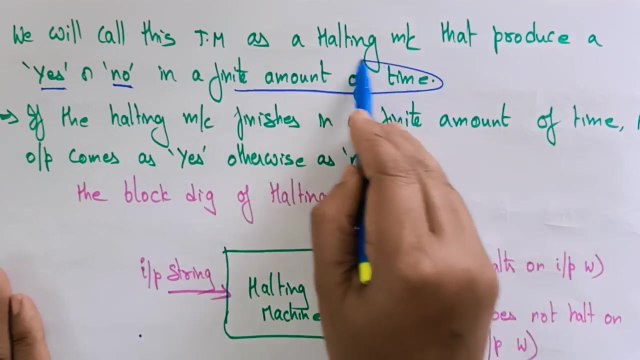 let us assume and then we will show it is contradicting itself. okay, now let's see how it is. so we will call this turing machine as a halting machine. so, whatever the mission we are taking, that is a halting machine. just call it. that produced s- either s or no- in a finite amount of time. 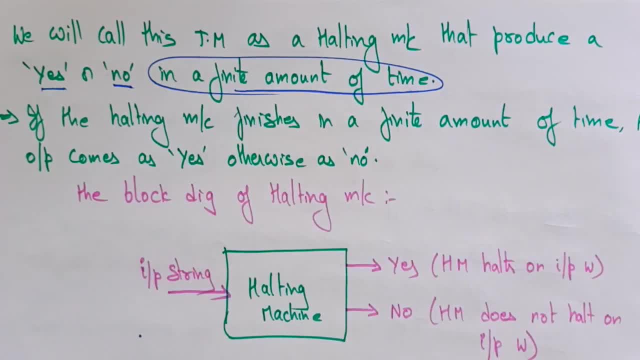 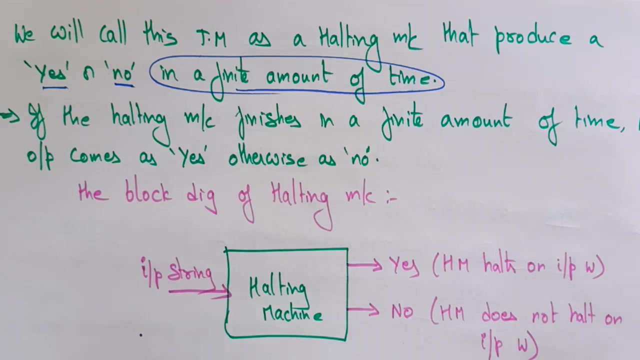 because i want the answer: answer in the finite of amount of time. it has to compute the given input string or it has to stop that given input string. so that is a problem i have to find out. so i am taking the halting machine that produce, either it can, two options, only, two answers. only it will give either it. 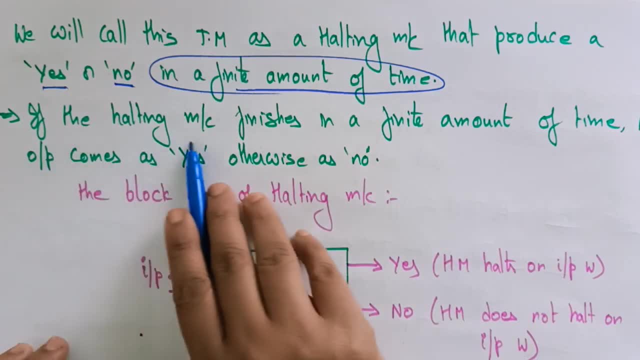 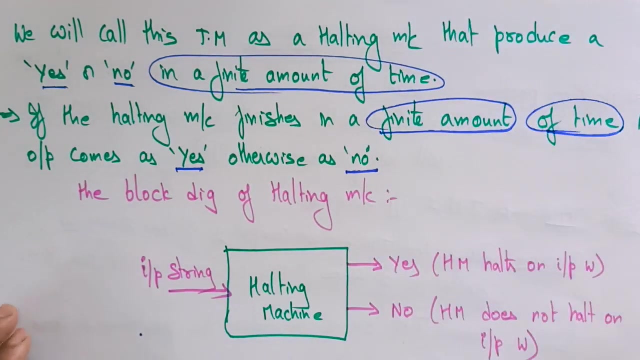 give s or no in a finite amount of time. so if the halting machine finishes a finite amount of time, the output comes as yes, otherwise no, that is a problem. so if the halting machine finishes in the finite amount of the thing here is that should be infinite amount of time, not is an. 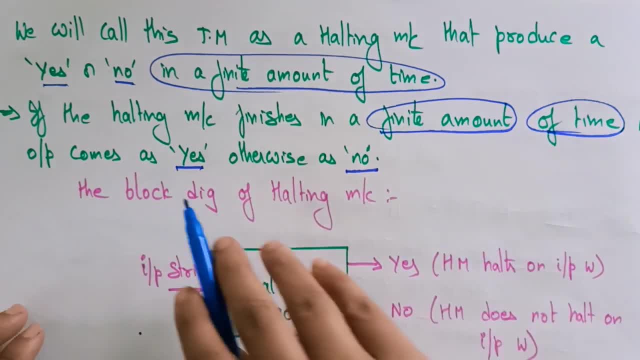 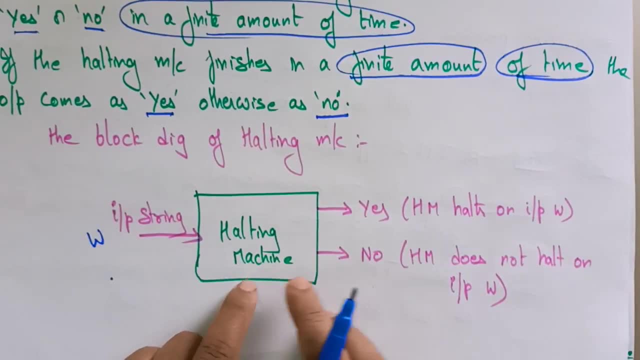 infinite amount of. so finite amount of time. the output comes as yes, otherwise no. so see, here in the block diagram i am given an input string, w. okay, now the halting machine is going to give an output either s or no. infinite amount of time. finite amount of. 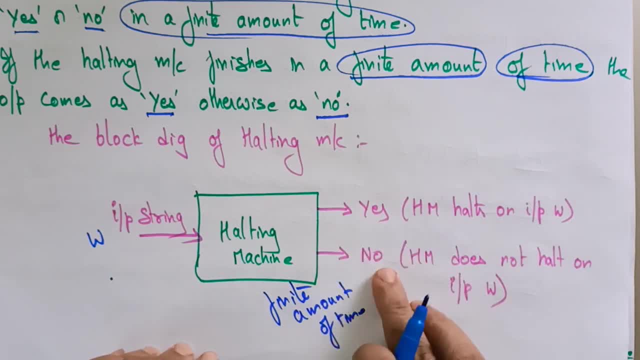 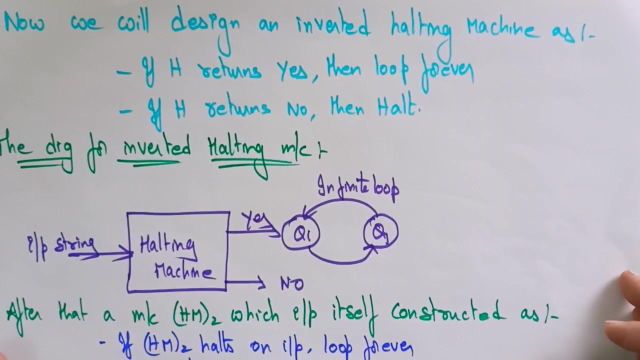 time time. so that may be the s or no. s means the halting machine halts on input w and a halting machine does not halt on input w. so that is about this, okay. so see, here now we will design an inverted halting machine. so whatever we are taking, just 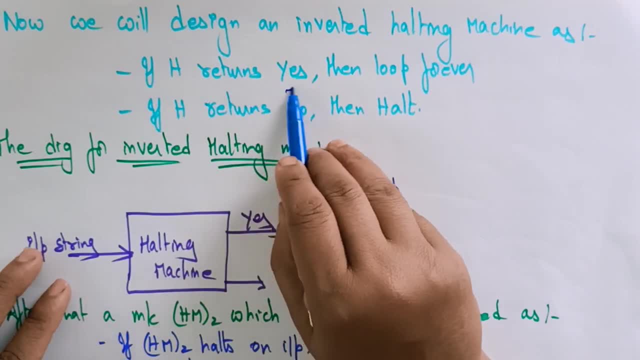 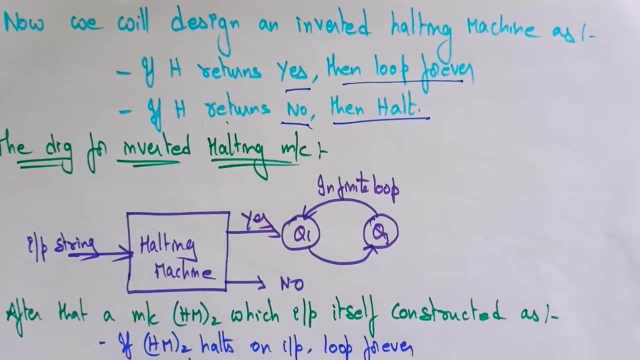 contradiction for that. so let's take halting machine returns s, then loop forever. halting machine returns no, then halt. so just we are taking the inverted or halting machine. these are the conditions for that. so the same way, the diagram for this inverted halting machine is: just, we are.